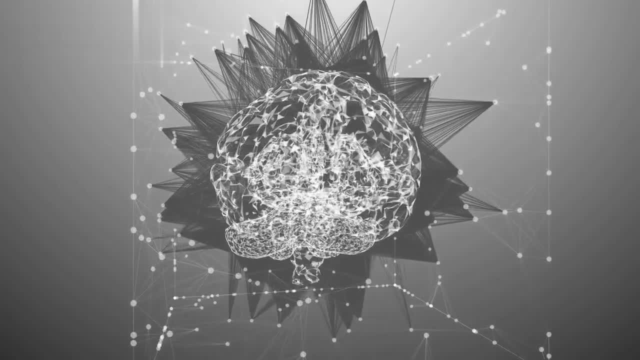 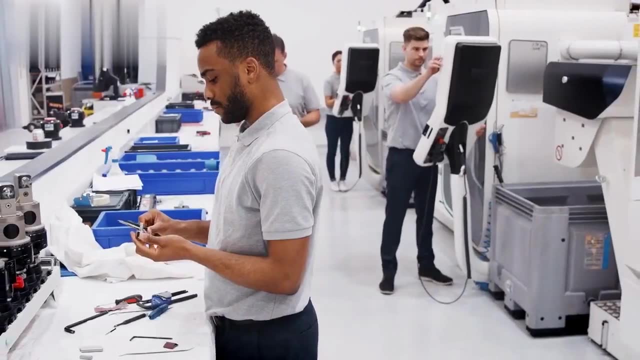 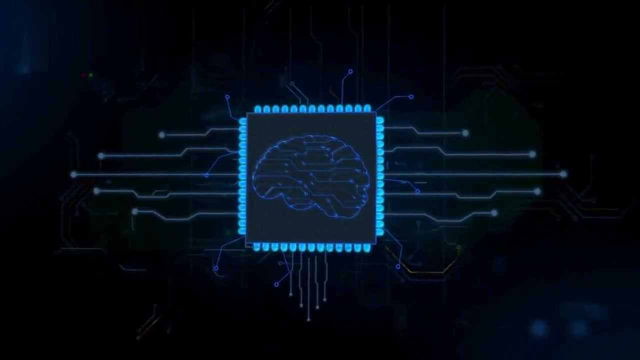 Welcome to our channel: Education in Smart Biomedical Engineering. Today, we're going to be talking about the basics of smart biomedical engineering. What is smart biomedical engineering? Smart biomedical engineering is a field of study that combines engineering, computer science and biology to create new technologies and devices. 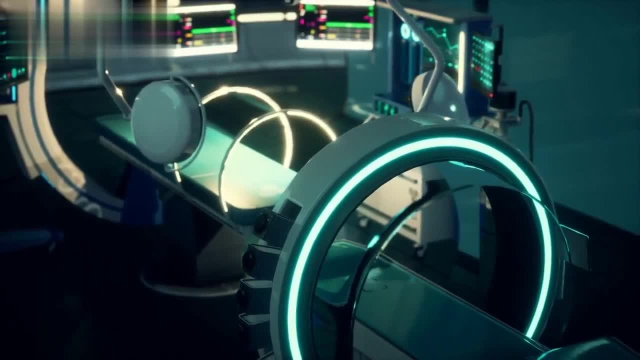 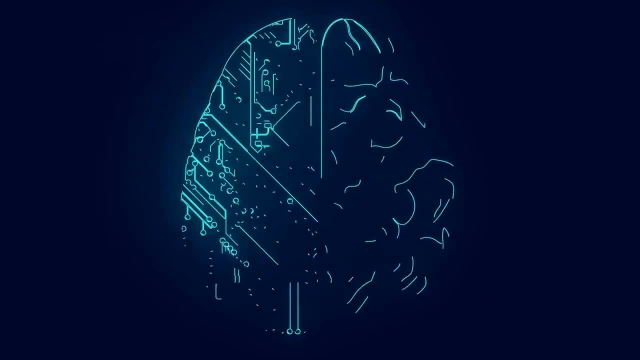 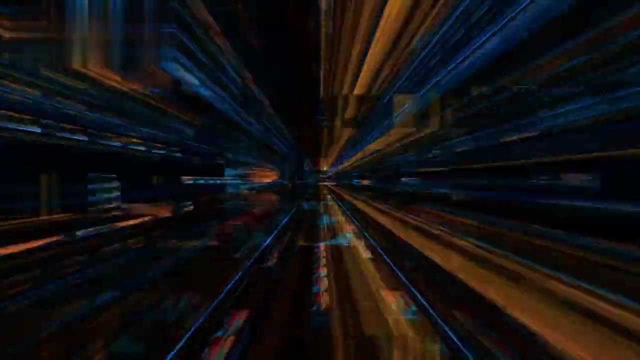 that improve human health. This includes things like artificial organs, medical imaging equipment and implantable medical devices. Advancements in Smart Biomedical Engineering. One of the biggest advancements in smart biomedical engineering is the development of artificial organs. These devices can replace or supplement the function of a human organ. 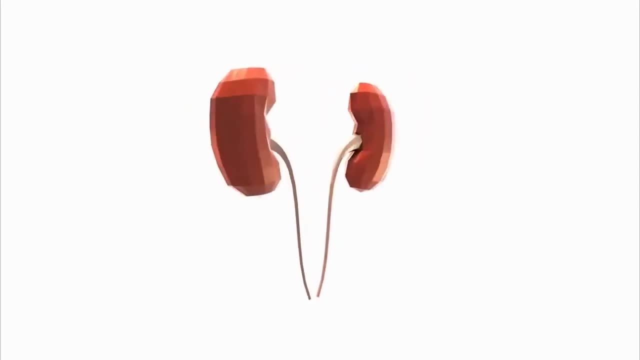 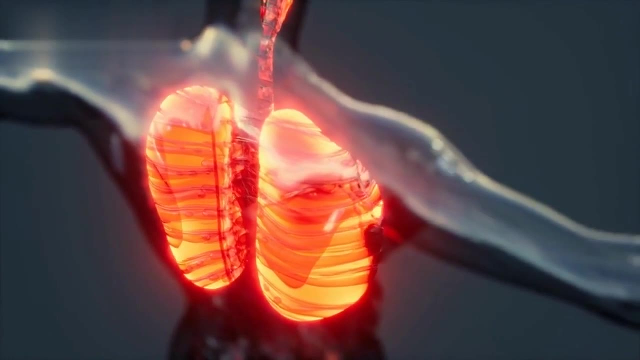 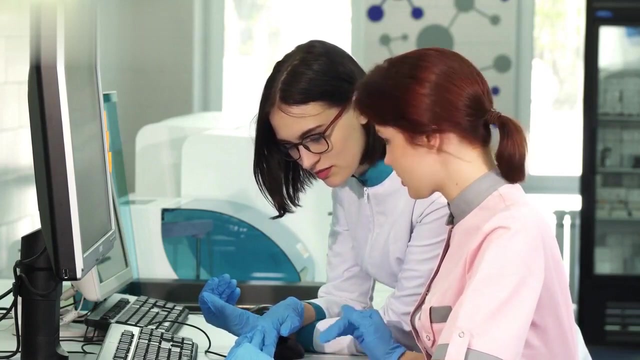 such as a heart or kidney, and can help extend the lives of people with chronic illnesses. Medical Imaging: Another important area of smart biomedical engineering is medical imaging. Engineers and computer scientists are working to create new imaging technologies that can provide more detailed and accurate. 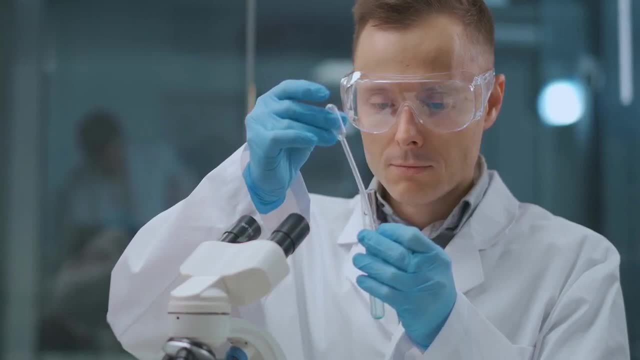 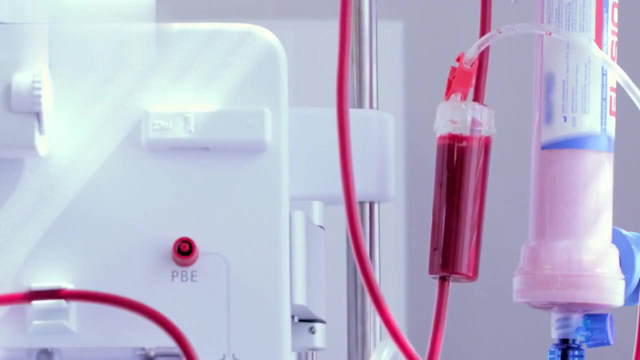 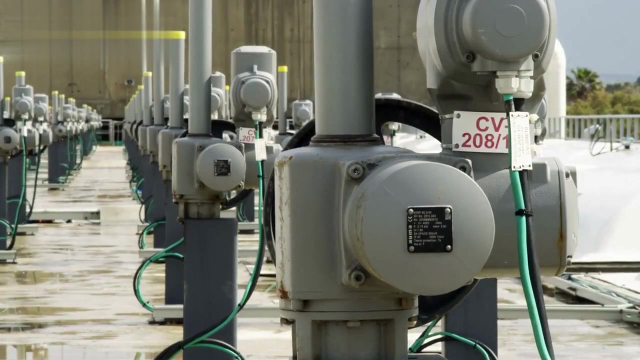 images of the body. This can help doctors diagnose and treat diseases more effectively. Implantable Medical Devices: Implantable medical devices are another important area of smart biomedical engineering. These devices, such as pacemakers and insulin pumps, can be implanted into the body to help treat chronic conditions. Engineers are constantly. 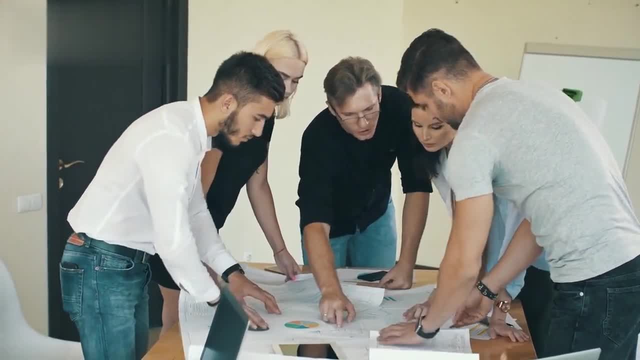 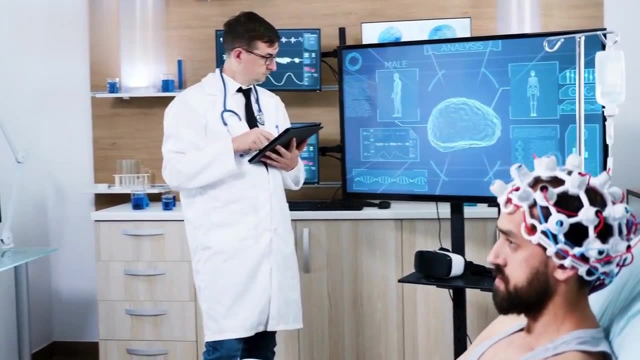 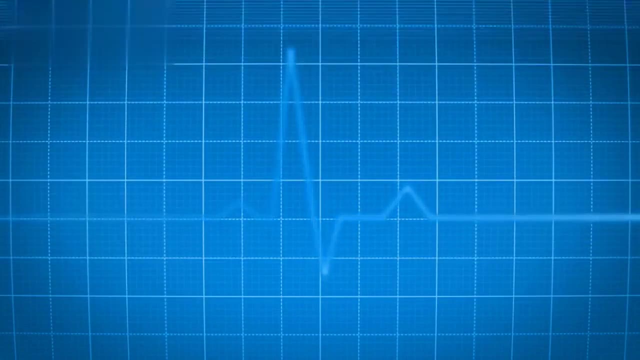 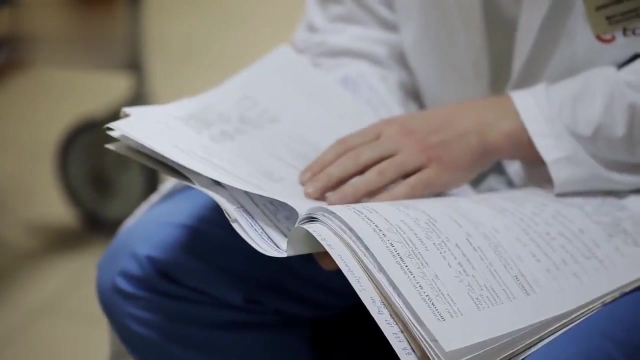 working to improve these devices. Biomedical Sensors: Another important aspect of smart biomedical engineering is the development of biomedical sensors. These sensors can be used to monitor various bodily functions, such as heart rate and blood sugar levels, in real time. This can help doctors and patients to better understand and manage chronic conditions. 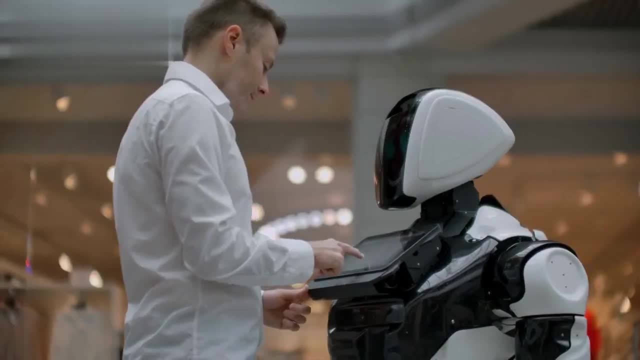 Robotics and Biomedical Engineering. Robotics is also playing a major role in smart biomedical engineering. This can help doctors and patients to better understand and manage chronic conditions. This can help doctors and patients to better understand and manage chronic conditions. Biomedical Engineering, Robotics and Biomedical Engineers. 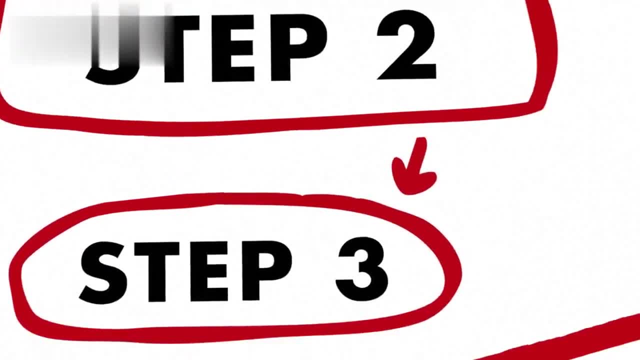 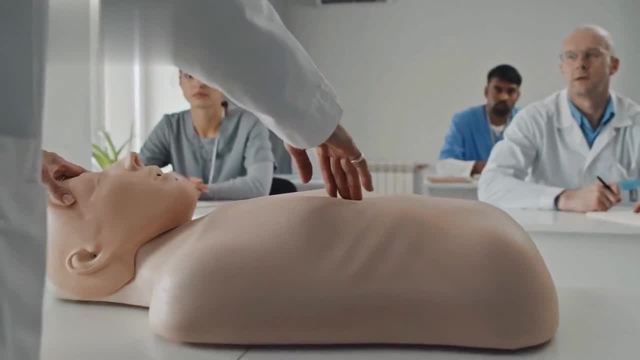 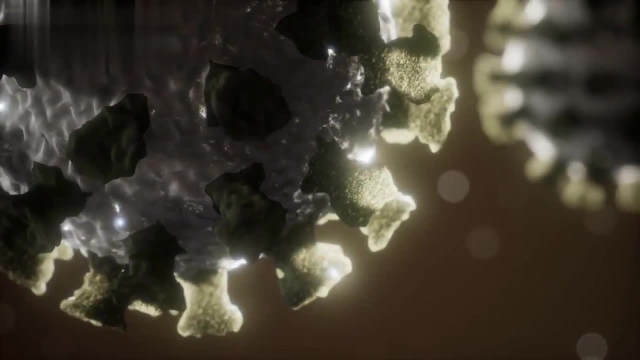 Robotics and Biomedical Engineers are developing robotic devices and systems that can assist in surgeries and other medical procedures. These devices can help to improve the precision and accuracy of these procedures, which can lead to better outcomes for patients. Personalized Medicine: Personalized medicine is another area of